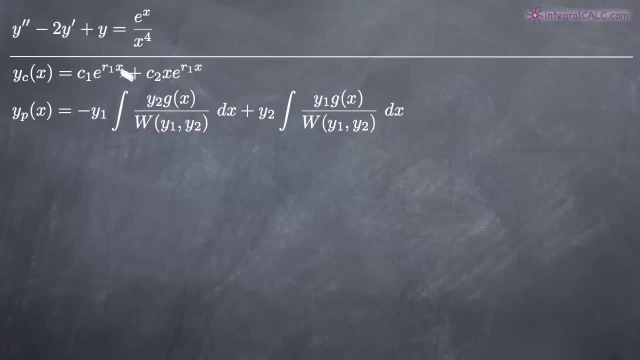 be to combine them or put them together, add them together. So the first thing we're going to do is find the complementary solution. Let me note one important thing When we're going to use the formulas that I've written here- not so much the complementary solution- 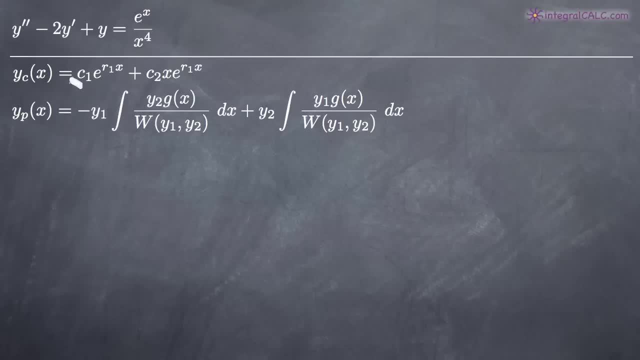 formula, but the formula for the particular solution. it's really important that we have a coefficient of 1 in front of our second derivative of y term. If you don't have a coefficient of 1, just divide that coefficient through the left and right hand side to make. 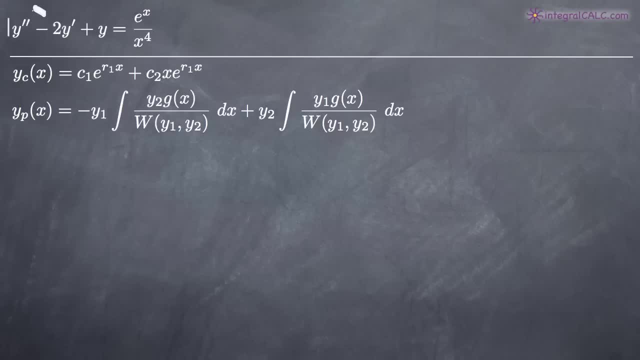 the coefficient 1.. And make sure you do that before you even get started with your problem, because this formula won't work unless you have that coefficient of 1.- 1.. So we do have a coefficient of 1.. So we'll go ahead and get started with our complementary. 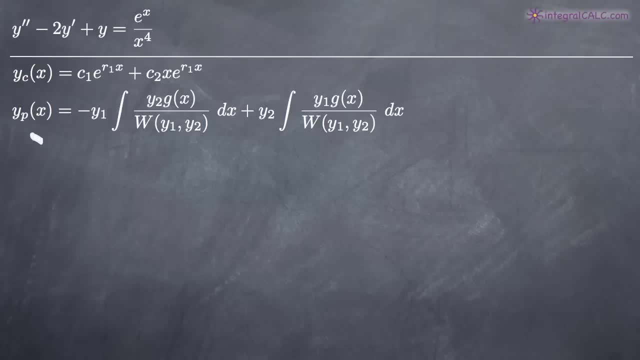 solution. And remember that to find the complementary solution, we're just going to turn the y's on the left hand side into r. So, because it's the second derivative of y, we have r squared minus 2 times r plus 1.. And we'll set that equal to 0.. We'll ignore the right hand side. 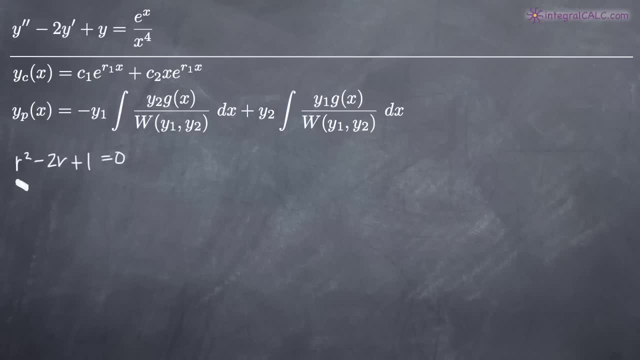 of our equation, for now We'll set it equal to 0.. And our goal is to solve for r. So in order to do that, we're going to have to find the complementary solution. And remember that to find the complementary solution we have to factor. We'll get r minus 1 times r minus. 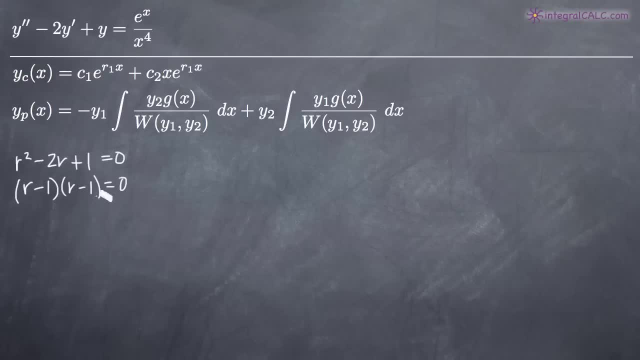 1 equals 0.. And you can see that we have two solutions, but they are identical solutions, So it's really just the same solution of r equals 1.. Which is why we've written here this particular complementary solution formula, which is the formula for the complementary. 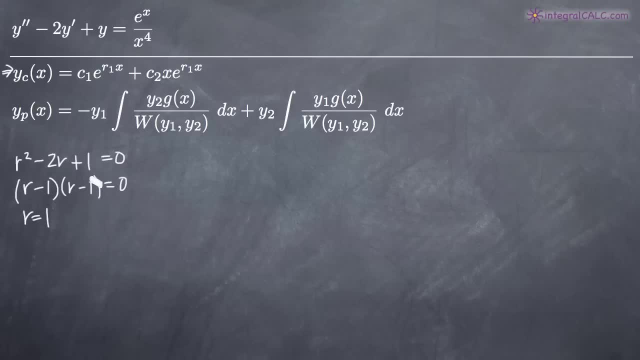 solution when you have equal real roots. Right, you have two roots, but they are equal, So. So we'll use that formula and we'll go ahead and write the complementary solution. So a complementary solution when both of our roots are equal to 1, will be- and I'm 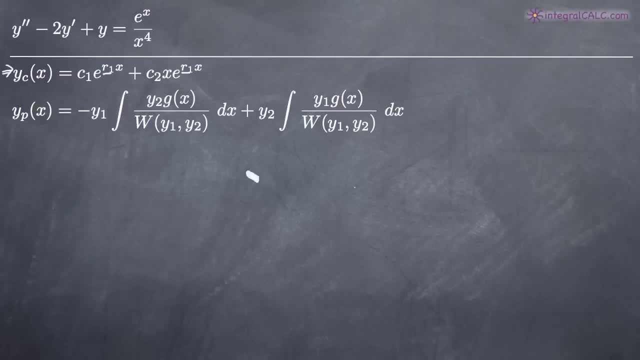 just going to give us a face as we go, because we'll need it. But the complementary solution will be c sub 1, which we always leave. We leave c sub 1 and c sub 2 alone. they're constants e to the 1x. 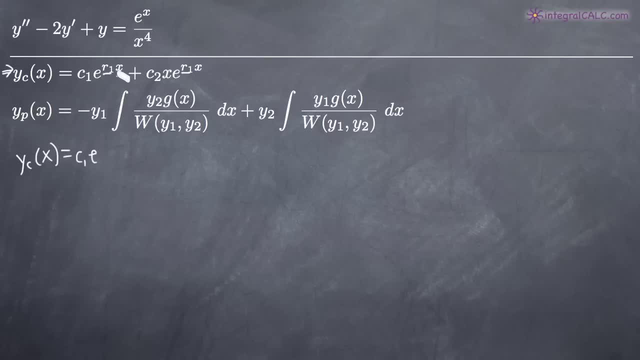 We'll be plugging in 1 for r sub 1.. We don't need to write 1x, we'll just write 1.. Plus c sub 2x again to the 1x. so we'll just write e to the x. 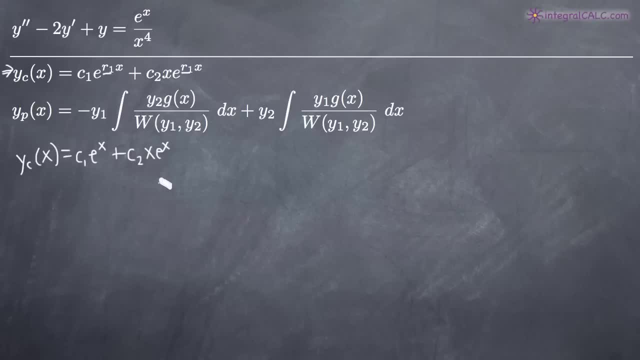 Alright, so this is our complementary solution. It's as easy as that. Now we can move on to the particular solution, But there's a couple of things that we need to do before we can start plugging things into our particular solution. Notice that we've got several components here that we don't know yet. 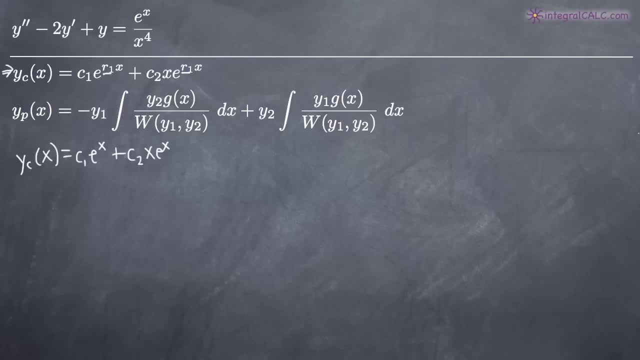 First of all, we have y sub 1 written here. We don't know what the y sub 1 is. It's written in here a couple of times. We also have y sub 2. that's included in the formula a couple of times. 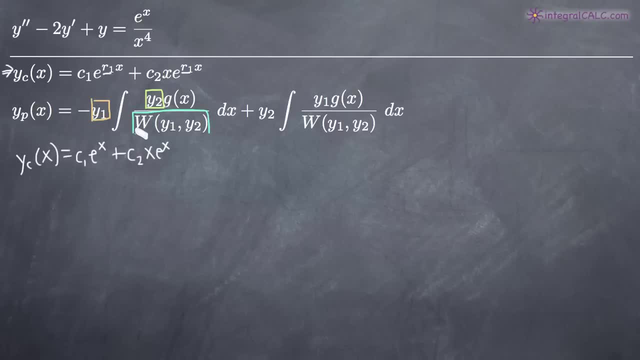 We have the Wronskian here of y sub 1, y sub 2, and we have g of x, none of which we've defined yet. So before we can go forward, we need to define those things Well. y sub 1 is going to be really easy. 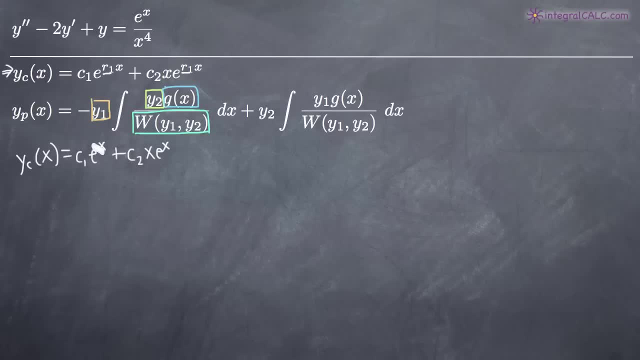 It's just whatever is attached to c sub 1 in our complementary solution but doesn't include c sub 1.. So e to the x is multiplied by c sub 1.. We're just going to leave that c sub 1 out and grab everything that's attached to it. 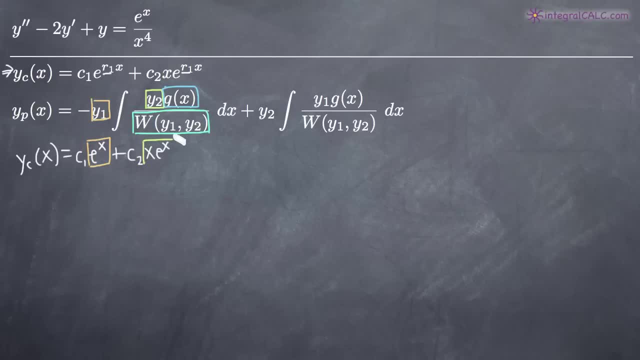 y sub 2, similarly will be everything that's attached to c sub 2 like this. So I'll grab that We now have both of those. g of x is going to be the right-hand side of our original second order differential. 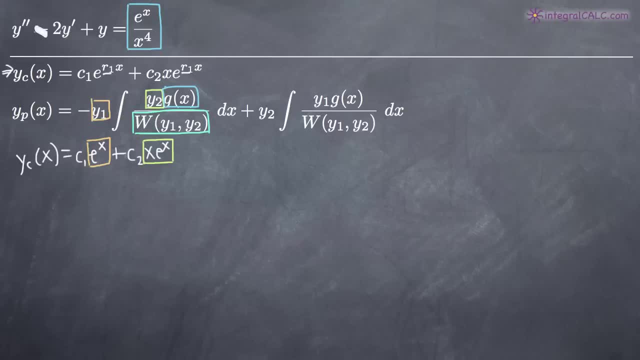 equation up here. So if we had to divide through to make the coefficient on the second derivative, 1, it would include whatever manipulation was there. So that's going to be g of x and then the Wronskian we're going to solve for right. 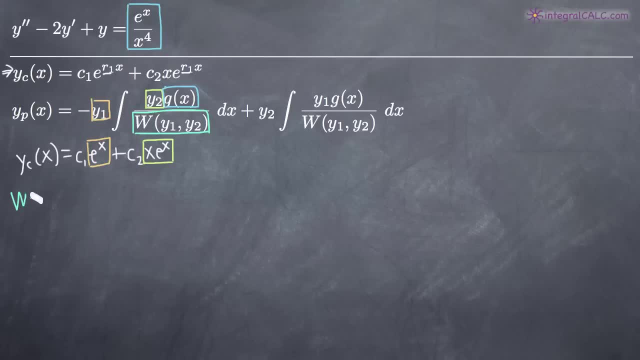 now using y sub 1 and y sub 2.. So our Wronskian is going to be equal to, and we'll draw a matrix here. What we're going to do is we're going to put y sub 1 and y sub 2 in here in the first. 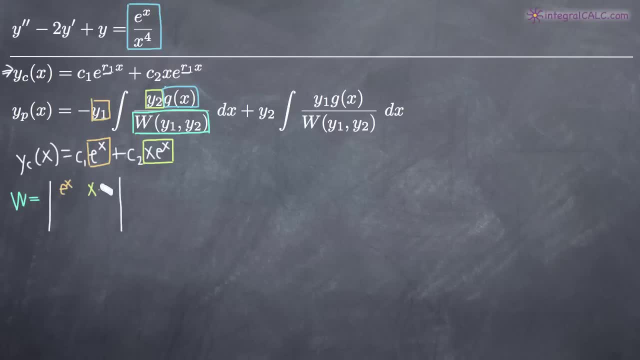 row. So y sub 1 e to the x and y sub 2 x e to the x. Then in the second row we're going to take their derivatives. So the derivative of e to the x is e to the x. Over here the derivative will be e to the x plus x e to the x which we use product. 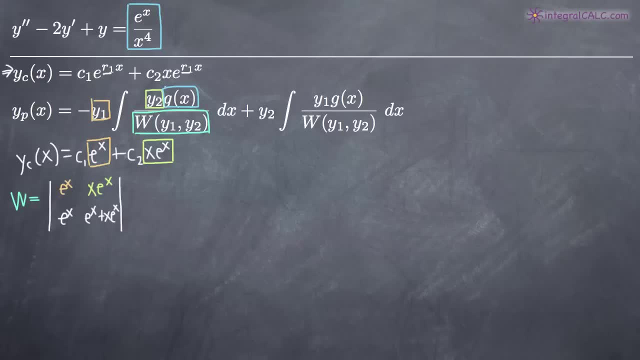 rule to find. So those are our derivatives, and now our Wronskian will be this first term here. So we'll multiply those together and we'll get e to the x times e to the x plus x, e to the x, and then we'll subtract whatever we get when we multiply these other two together. 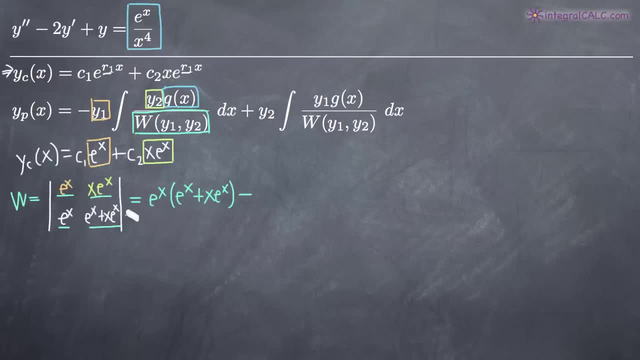 and we're multiplying on the diagonal. So we'll get here e to the x times x, e to the x, and it's as simple as that. Just remember that you're multiplying first this way and then you're multiplying this way, Then subtracting, then multiplying this way. 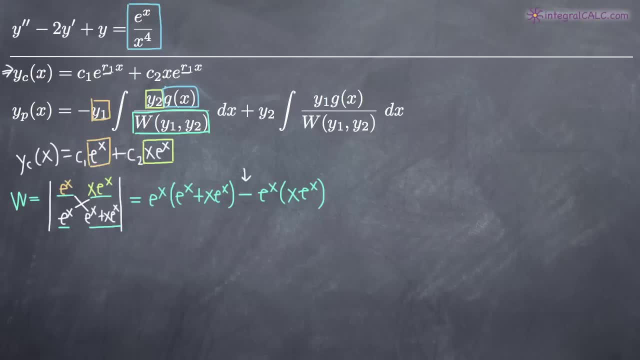 Those are really the three things that you have to remember with the Wronskian. So now all we have to do is simplify this as much as possible to find the Wronskian that we're going to plug into the formula for our particular solution. 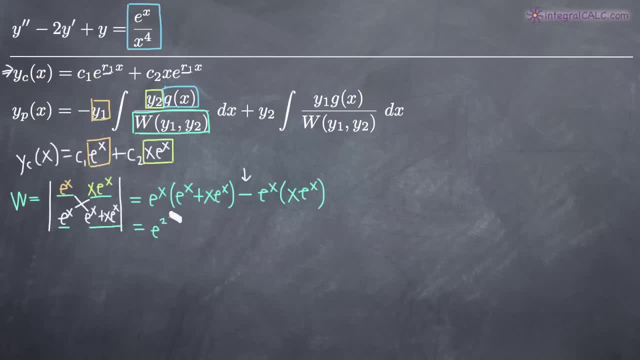 So e to the x times e to the x will give us e to the 2x plus x, e to the 2x minus x, e to the 2x. So, as you can see, the second and third term here are going to cancel and we're just left. 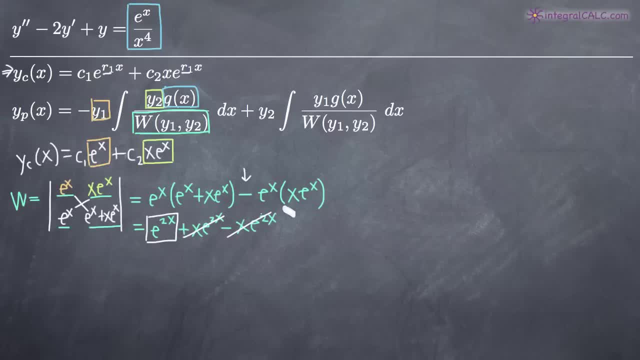 with e to the 2x. So that's going to be our Wronskian. So now we've got all four components and we can go ahead and plug those in to the formula for our particular solution. So y sub p for particular of x will be equal to- don't forget to include this negative. 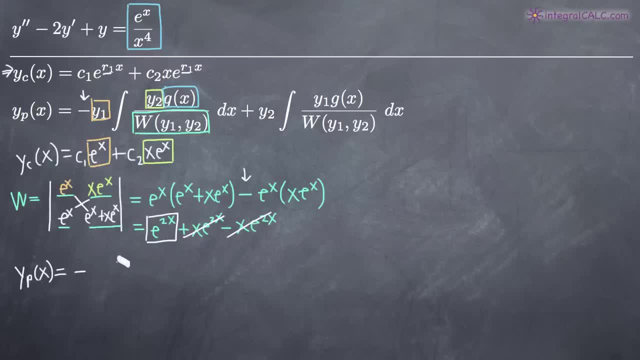 sign. it's really important. So we have the negative sign and then y sub 1, which we already know to be e to the x, plus the integral of y sub 2, so x, e to the x times g of x, e to the x divided by x to the fourth. 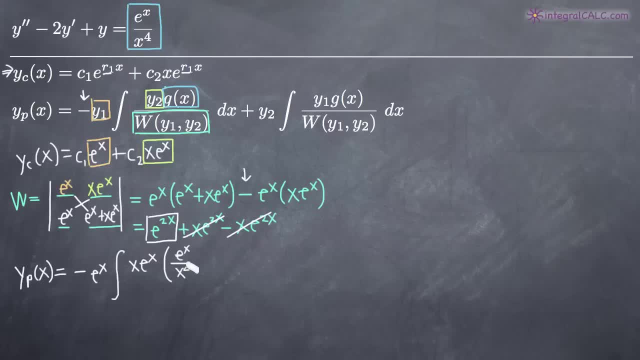 all divided by the Wronskian, which we know is e to the 2x, dx. And then our second integral here is going to end up looking similar. We just have y sub 2 on the outside times, dx, So that's going to be e to the x. 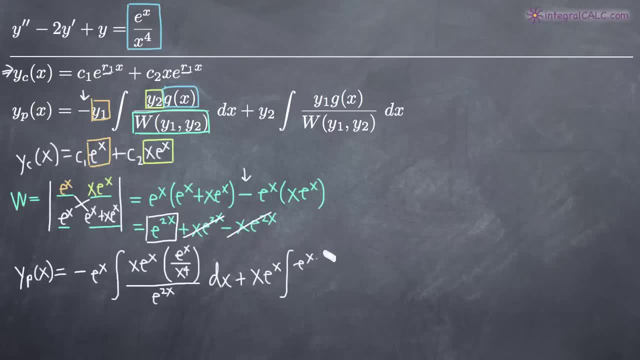 And then the right hand side of our original differential equation, all divided by the Wronskian e to the 2x dx. So that's it. We just plug in all of these components to our particular solution formula, and now it's just a matter of simplification. 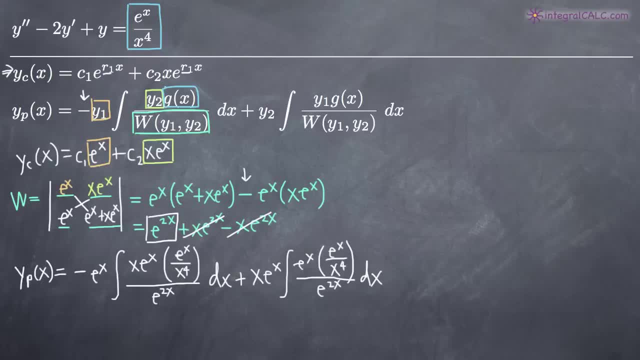 So let's start looking at a couple of these things. This is going to simplify for us fairly quickly, So we're going to plug in all of these components. First of all, we can see here in the numerator of our first integral, we have e to the x. 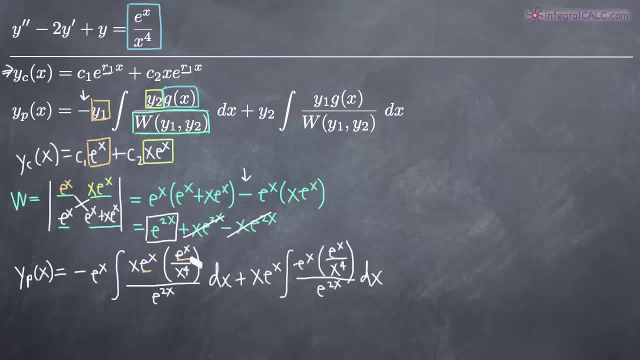 times e to the x, which we know will become e to the 2x. Those are in the numerator of our fraction here and we also have an e to the 2x in our denominator, so those three will cancel with one another. We can see over here in the second integral that we have the same thing. 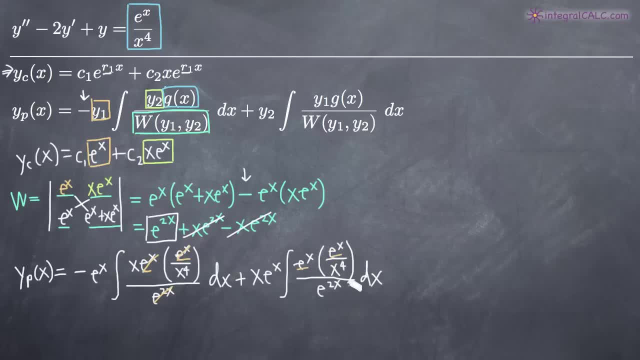 We have e to the x, times e to the x in the numerator, which will give us e to the 2x in the numerator, which will cancel with e to the 2x in the numerator. So those three are going to go away. You can also see that in our first integral we have x in the numerator and x to the fourth. 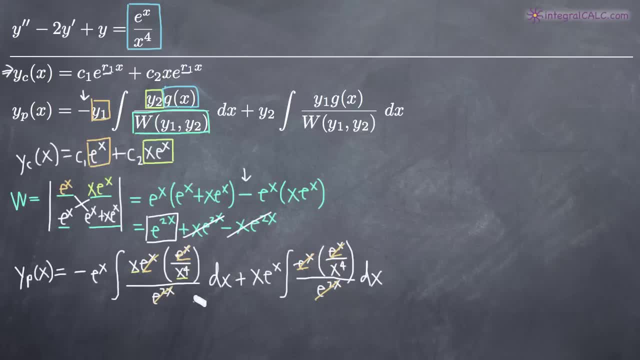 in the denominator. So this x is going to go away and we're going to be left with x to the third power here. We'll write this out again in a second. But x to the third power you can see in the second integral, we're just going to be left. 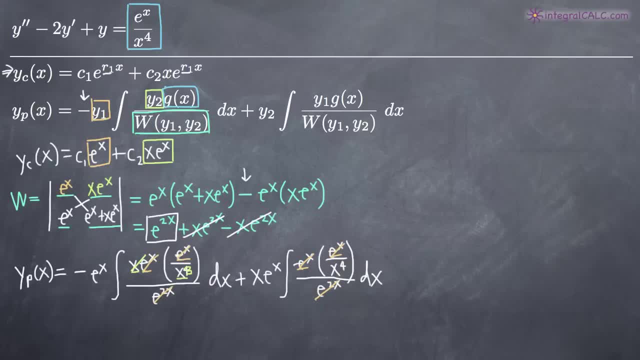 with x to the fourth. So let's go ahead and clean this up a little bit. y to the particular is equal to negative e to the third power. x to the third power is equal to negative e to the x times the integral of 1 over x. 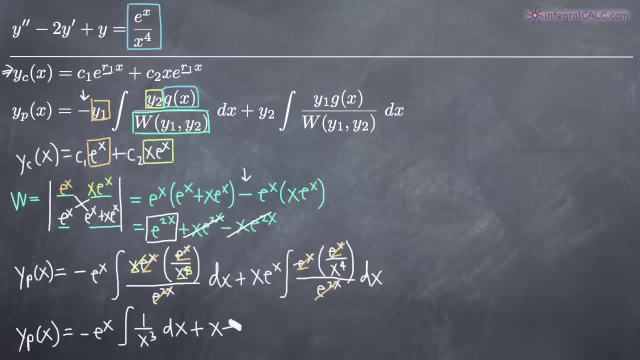 cubed plus x, e to the x, times the integral of 1 over x to the fourth, dx. What I'd like to do at this point is change those 1 over x cubed and 1 over x to the fourth into negative exponents. 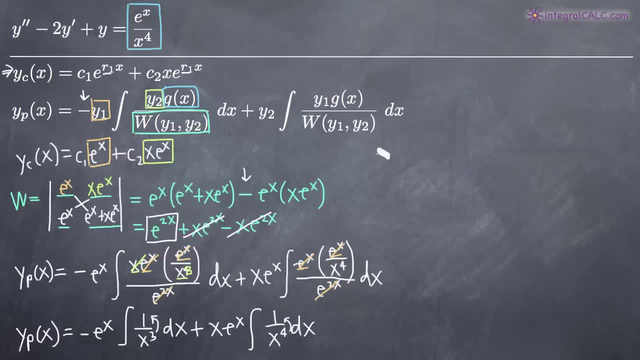 Remember that we can move these to the top and just make the exponents negative. That'll make our integration really easy. So the particular solution is negative: e to the x times the integral of x to the negative 3 dx plus x. e to the x times the integral of x to the negative 4 dx. 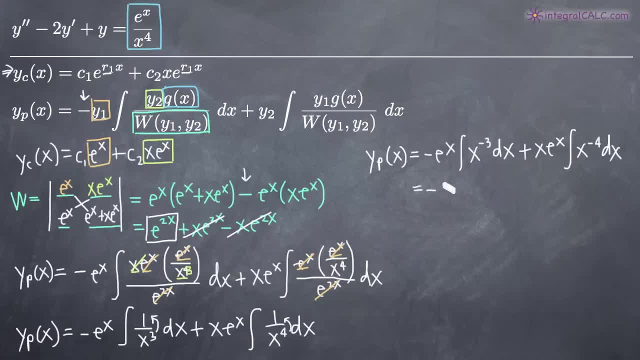 Okay. so now we can go ahead and integrate really easily. So we have negative e to the x times 1 over negative, 2, dx. Okay, So we have x to the negative, 2 plus x. e to the x times 1 over negative, 3 x to the negative. 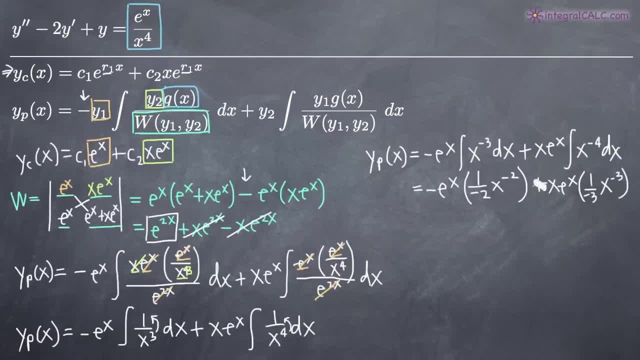 3.. One thing I want to note at this point: normally, when you take an integral, remember that you have to add the constant of integration, right, You always integrate and then you add a plus c to account for that constant that could have been there. 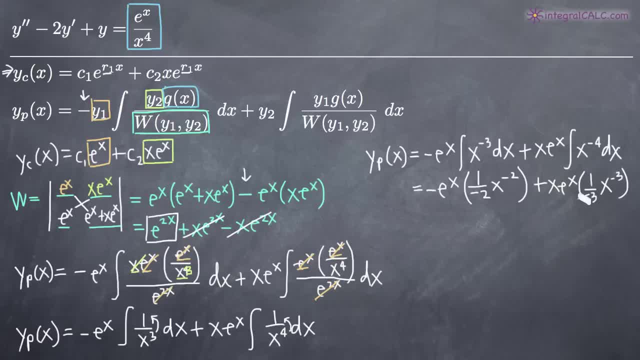 Well, in this particular method, when we're using variation of parameters and this solution has this formula for the particular solution, you actually don't have to add the constant of integration, because when you go and put this particular solution back with the complementary solution, those constants just end up canceling. 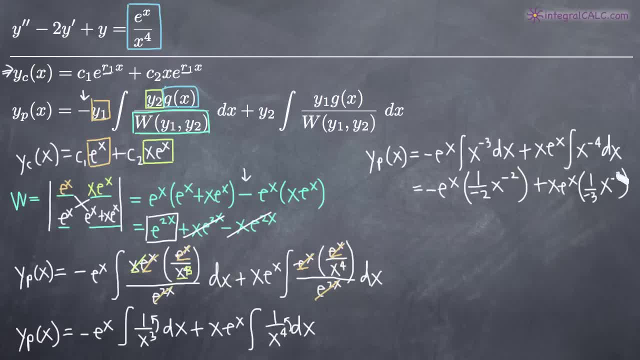 I'm not going to spend time in this video proving how they cancel, but needless to say, they'll cancel out every time, so you don't need to include them, unless your professor specifically asks you to include them, because they'll go away in the end. 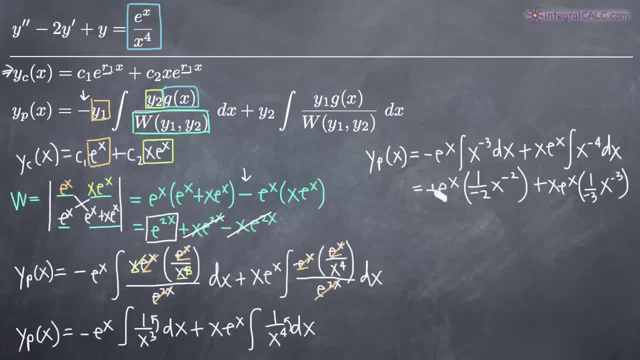 Okay, So now you can see that we've got a negative sign here and a negative sign here that will cancel each other out and become positive. This x to the negative 2 is going to move to the denominator and become x to the positive 2 in the denominator. 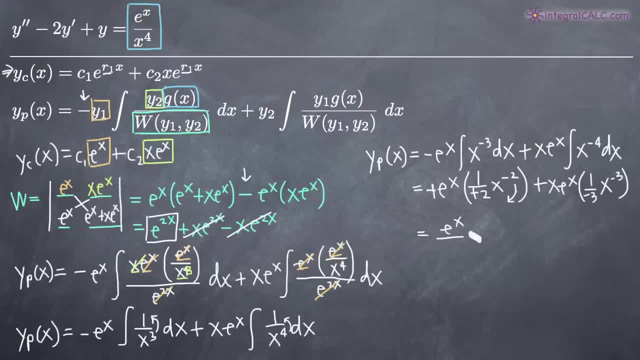 So we'll just be left with e to the x over 2x squared. Then over here in our second term we have a negative sign there in our denominator, so we'll say minus. Then we'll have x- e to the x in the numerator all divided by 3x cubed, because this x cubed. 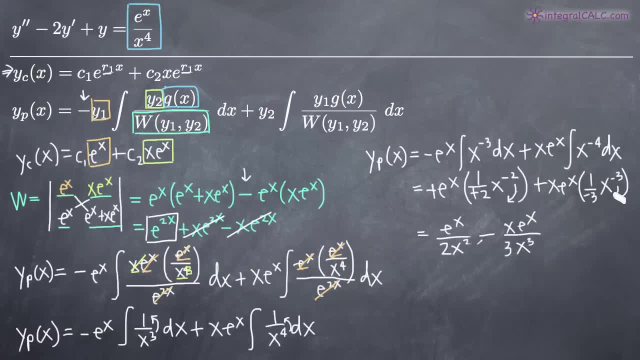 moves to the denominator as well. So there's a couple of things here we can do to simplify. First of all, we can cancel this x and this will become x squared. So let's go ahead and write that out: e to the x over 2x squared minus e to the x over 3x squared.